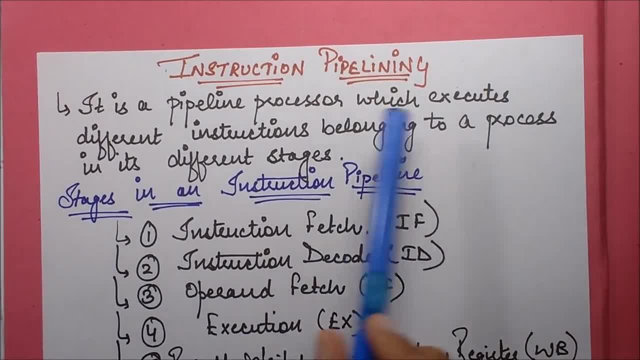 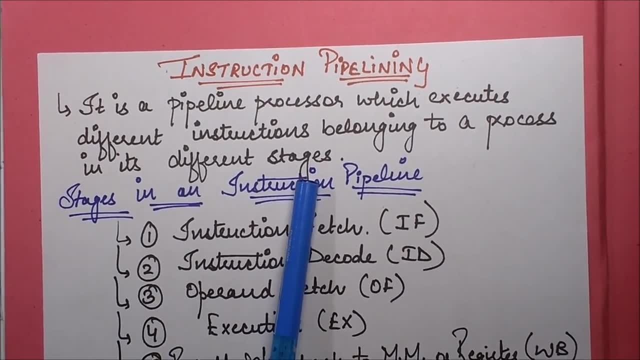 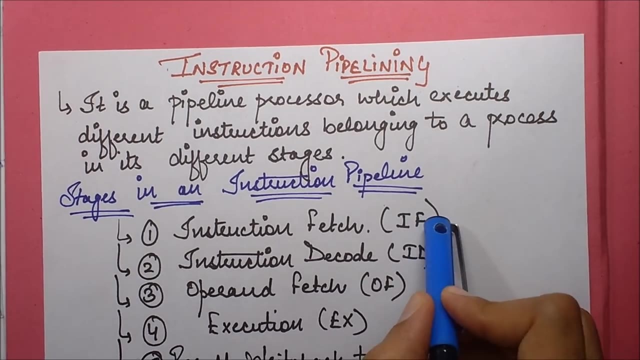 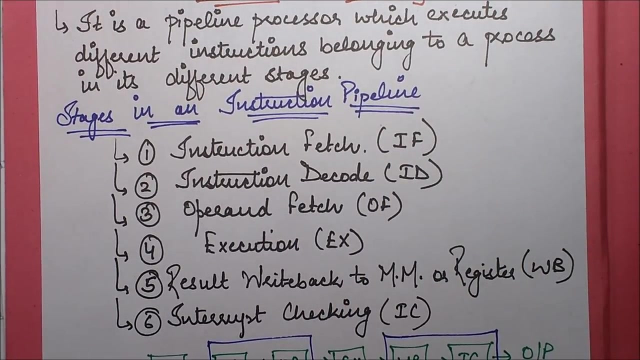 is a pipeline processor which executes different instructions belonging to a process in its different stages. fine, so an instruction is executed in its different stages. so the stages in an instruction pipeline are: what instruction fetch first you fetch that instruction, fetch that instruction. now, that instruction can be, can be in any form. for example, that can be in that can. 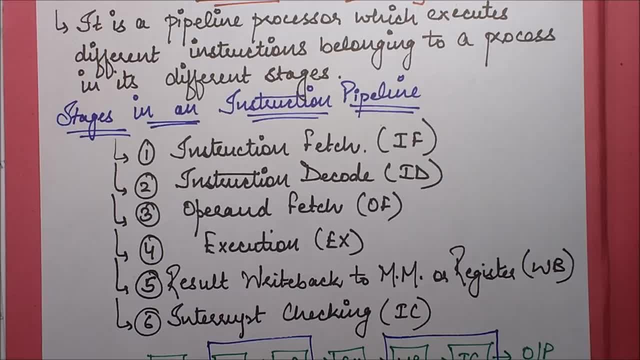 have any code of its straight so you can say: the instruction was add something, something right, so that is instruction fetch. then you decode it. you decode by decode you mean: what is the, what is the meaning of that? add instruction. you, that pipeline processor sees what is the decode, what is the code corresponding to. 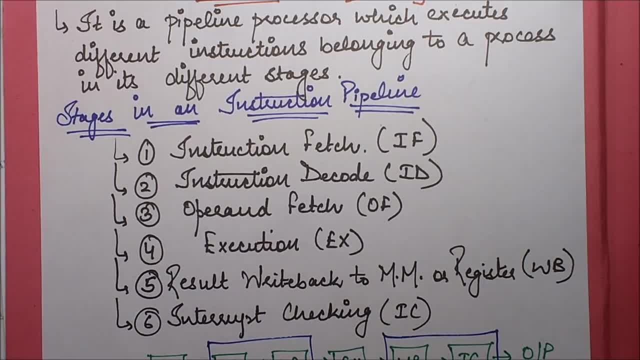 add. then next comes the operand fetch, 9 operand fetch. what do you do if it was a: add a, b? then you fetch the contents of a and b. so that is operand fetch. you fetch the operand on which the operation needs to be performed. then is the execution: you execute that operation. 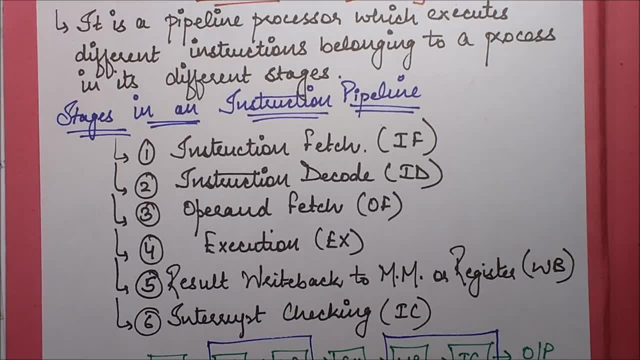 then resolve right back to main memory or register. you write back or store the results. and finally, is the interrupt checking. you check if there is some any interrupt or you need to do something else. so that's all is this? so if you represent this with the help of log diagram, 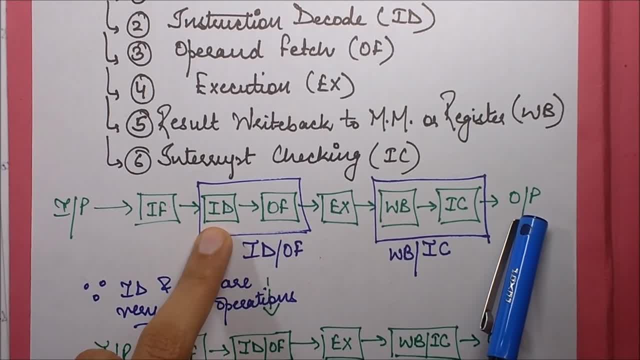 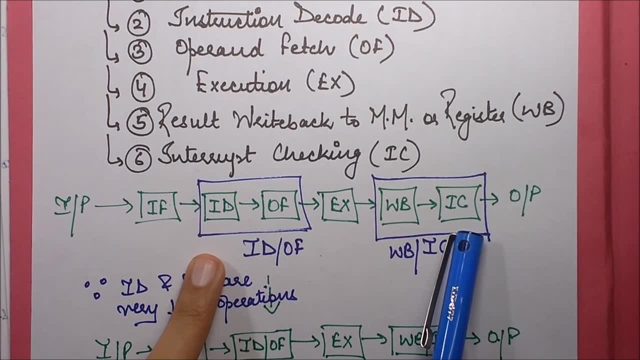 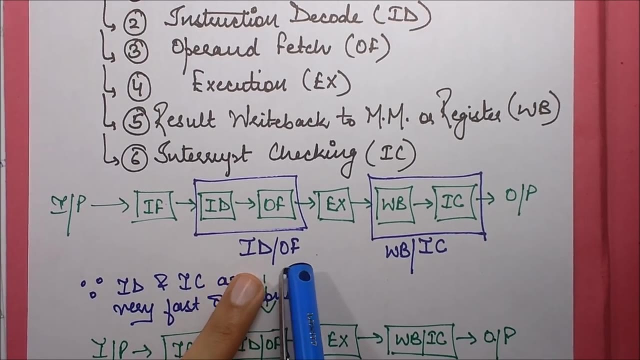 you represent it like this. now this instruction decode and write back operations are sorry. instruction decode and ic- ic was interrupt checking- are very fast operations. therefore they are clubbed in this manner. so instruction decode and operand fetch are clubbed together, and write back and interrupt checking are clubbed together. so we have a four stage pipeline system. 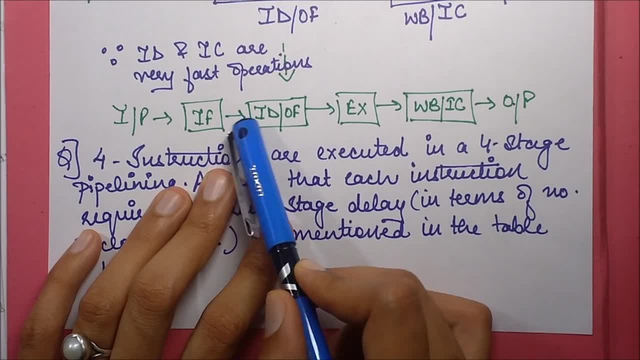 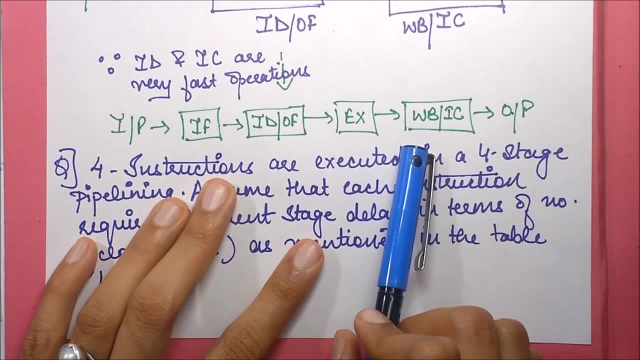 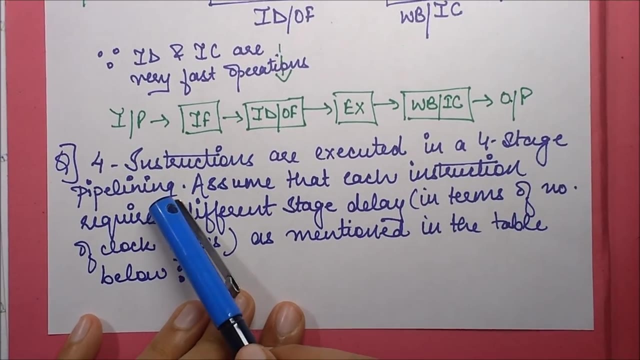 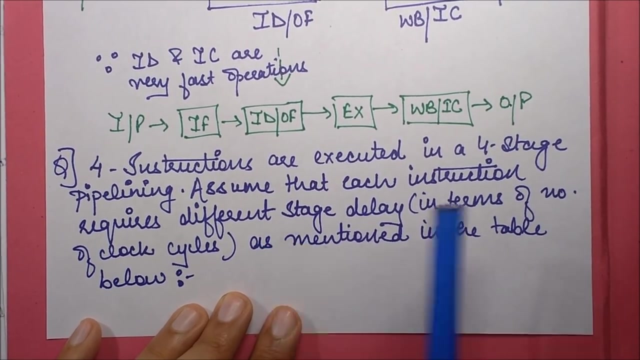 as the standard, which is this: instruction fit id slash of ex wb slash ic right. so let's quickly see a numerical on the basis of the same. we have four instructions are executed in a four stage pipelining. assume that each instruction requires different stage delay. so all the stages- let's say if there were four stages, t1, t2, t3, t4- are the 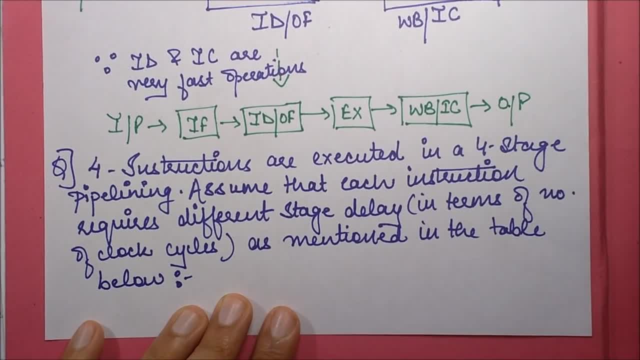 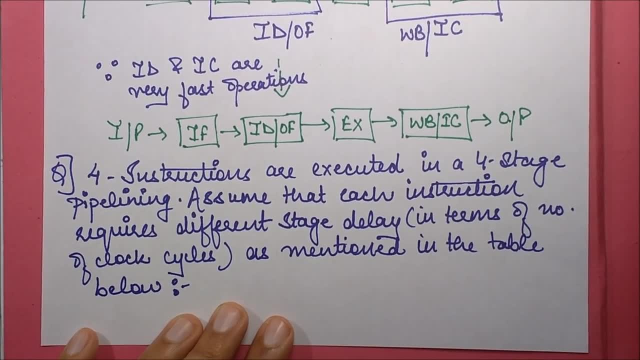 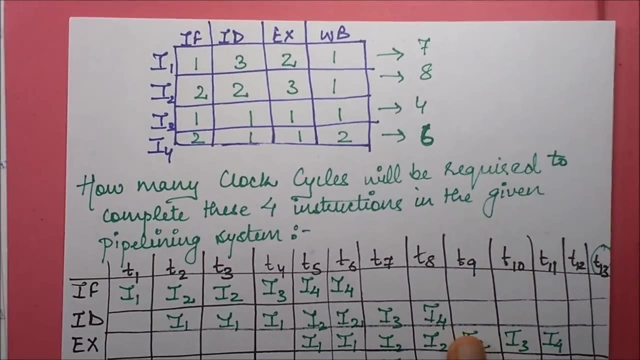 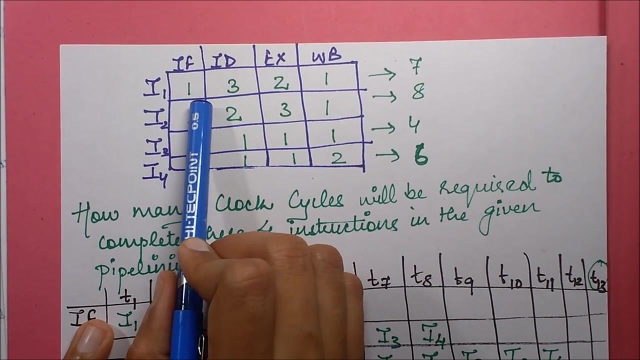 stage delays, as mentioned in the table below, now that you have been given a table which mentions different stage delays of all these four instructions. so there, there are four instructions and there are four stages and you have this table corresponding to it. so these are the four instructions, these are the four stages. so instruction one takes this much time in its 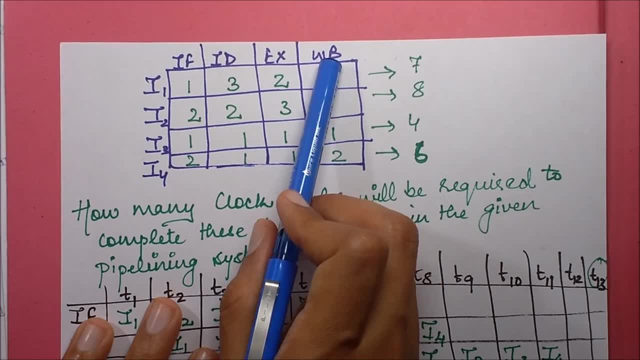 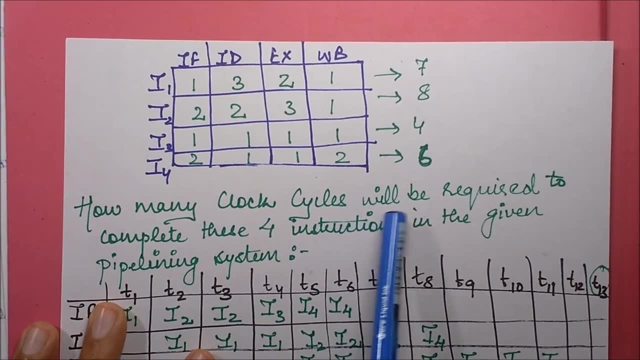 first stage, this much in second, this much in third, this much in fourth. similarly is given for i2, i3 and i4. now you need to find that how many clock cycles will be required to complete these four instructions in the given pipelining system? now, since they are not, 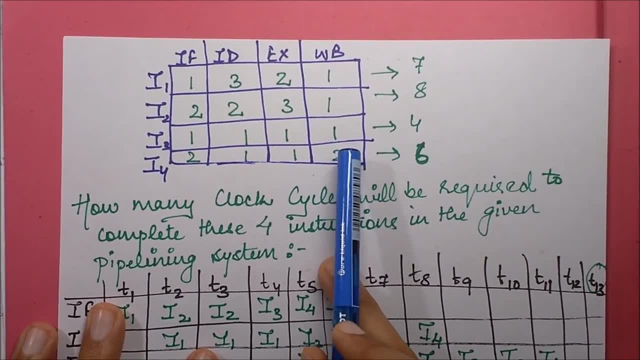 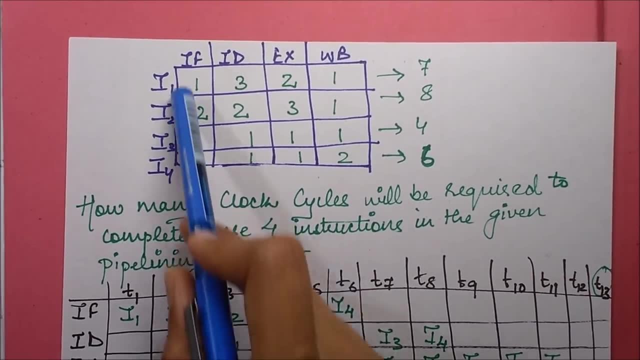 what you can say. they are not symmetric, the timings are not symmetric, so you'll have to manually draw the table and check what are the minimum clock cycle times in which you are able to complete all these four instructions. so what is the procedure? the procedure is very simple: just draw four. 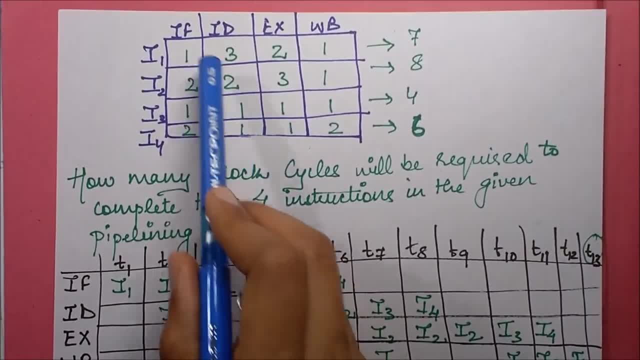 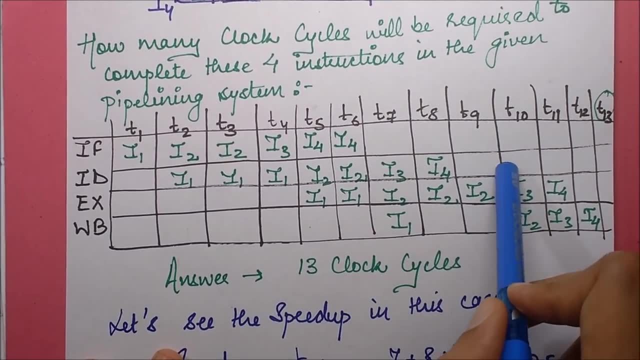 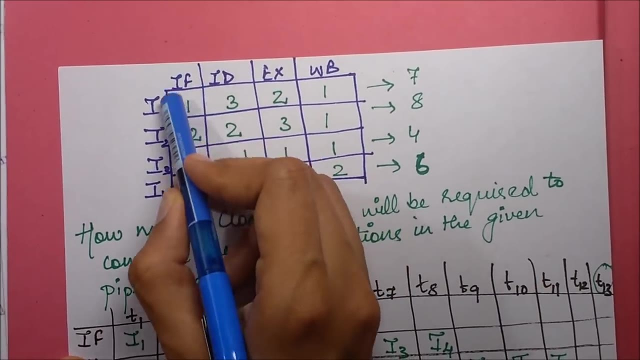 stages over here because we had four stages in this system. so we had four stages. we have drawn them over here and then we just keep on adding the clock cycle times over here till we end end up executing all the instructions, right? so in the first instruction fetch we know i1 takes only one clock cycle time. so i1 is only 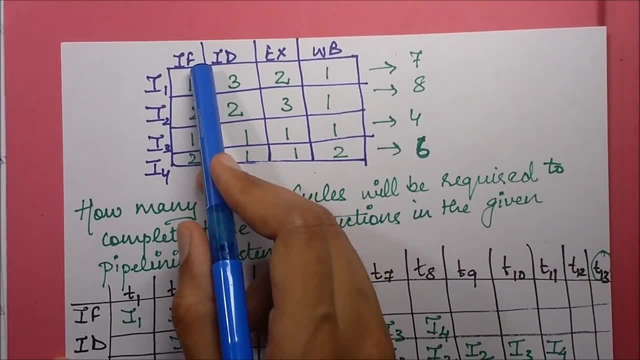 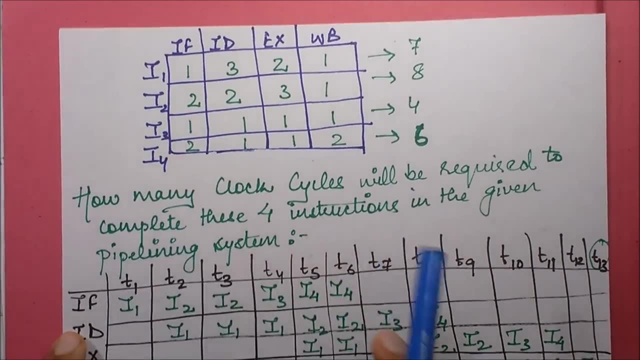 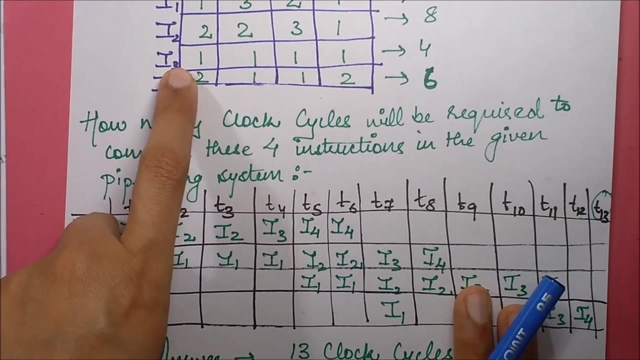 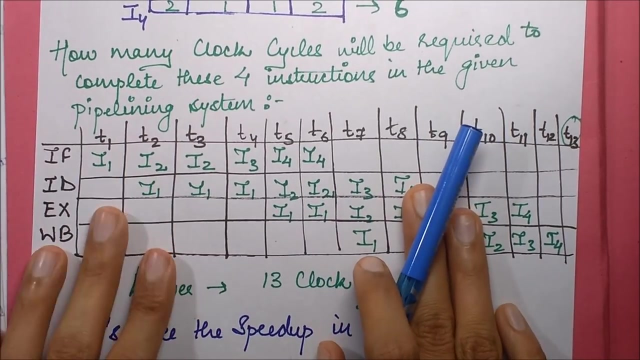 written once over here. then i2 in its if takes two. so we have two clock cycles for i2 instruction. so we just wrote i2 i2 twice in instruction, fetch right. then i3 similarly has one. so we wrote i3 once, and then i4 has two. so we wrote i4 twice. so now instruction. 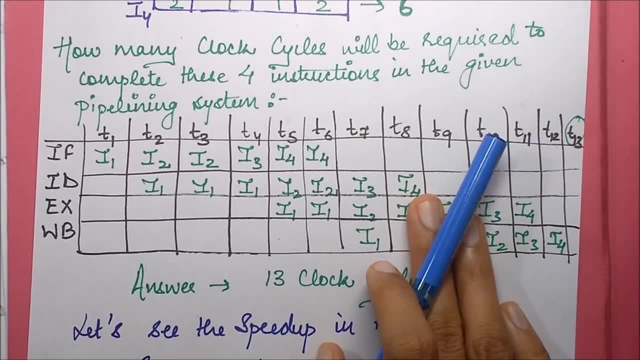 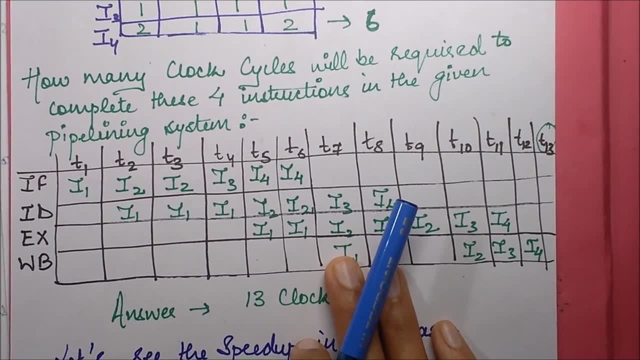 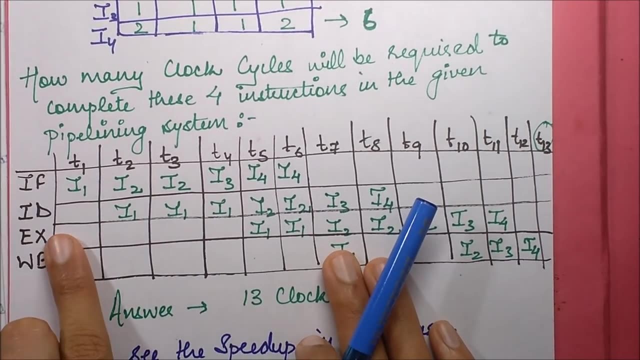 fetch is basically, uh, independent of all the other stages, and instruction decode as well. so instruction fetch and instruction decode can be executed without any delay. what do i mean by it? i'll just explain in a few minutes. so if this is clear, we move on to the next stage. after i1 is 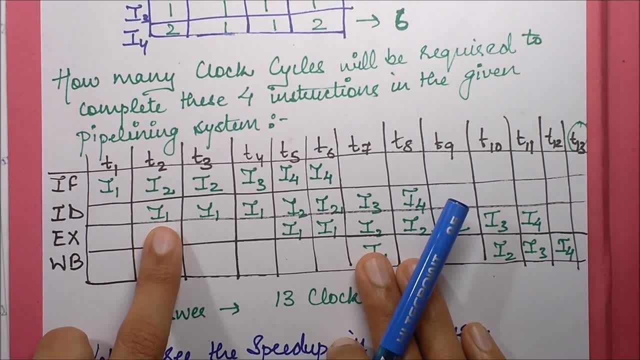 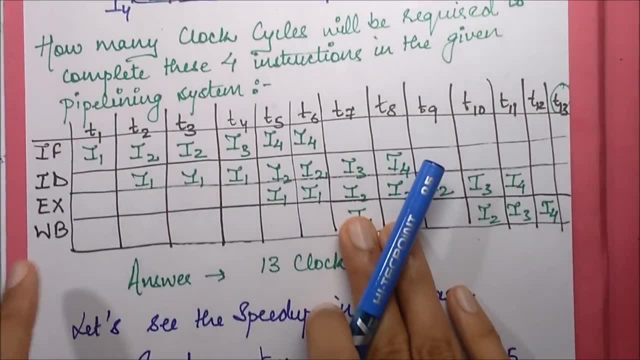 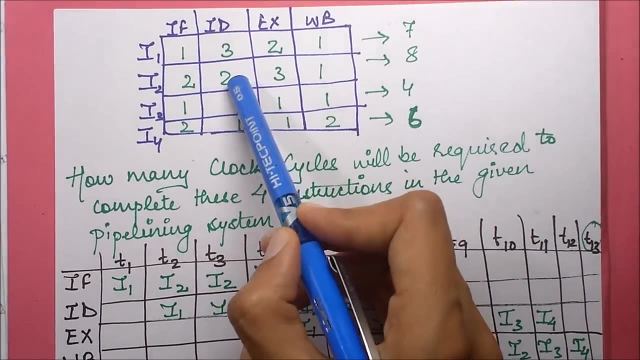 complete with it. with its first stage it will move on into its second stage. so i1 in its id stage, instruction decode stage, takes three clock cycles. so i1 will be written thrice i1, i1, i1. right now i2 will be taking how much time? it will be taking two clock cycles. so i2, i2, then i3 takes one, i3, then i4 takes. 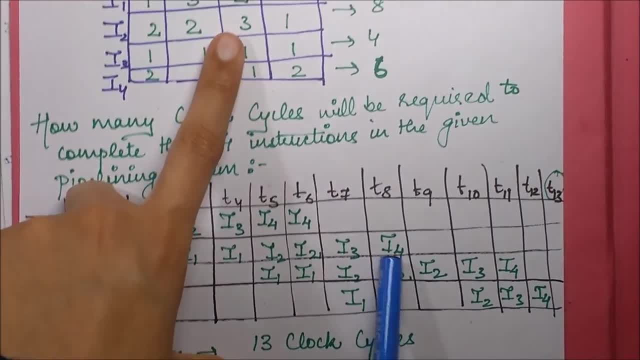 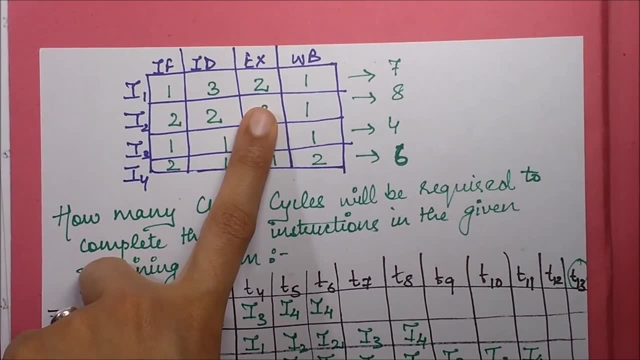 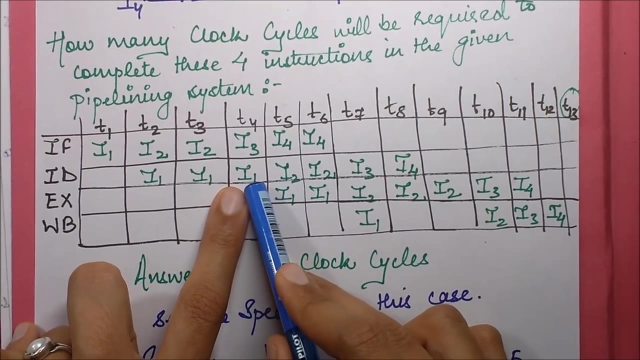 one i4, then after that in execution phase, after instruction has been decoded, can be executed, and i1 takes two clock cycles for execution. so after i1 has been decoded, only then, after i1 has been completely decoded, only then its execution will start. note: i didn't start. 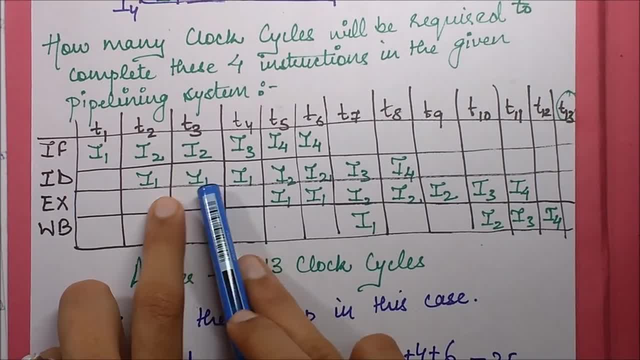 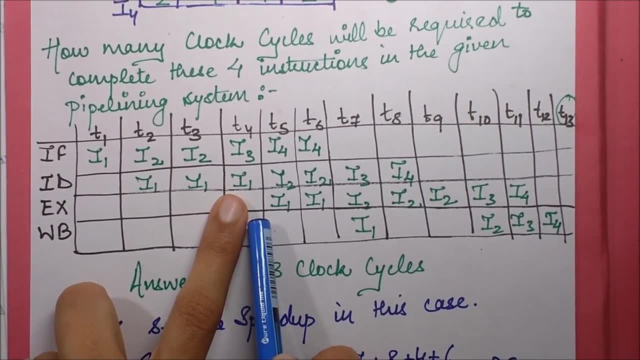 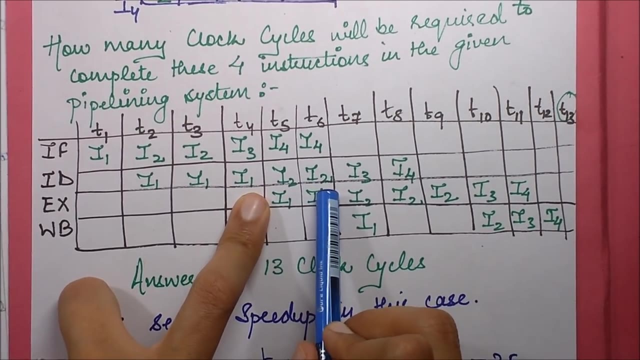 the execution from here, because i1 has not been completely decoded till here. it has been completed. it has completed its id phase over here. so now it takes how much time in execution. two clock cycles. so we wrote i1, i1 twice over here. now, similarly, i2 has been decoded till here, so i2 takes how. 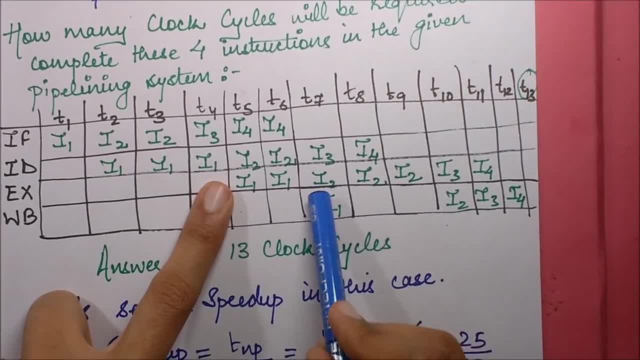 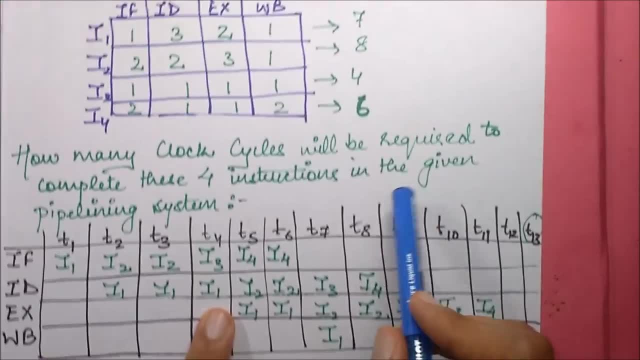 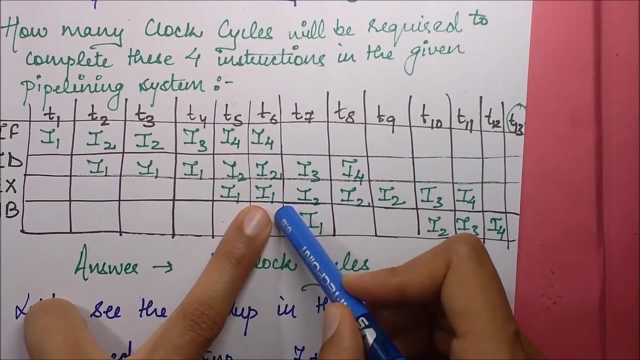 much time. it takes three clock cycles for execution. so i2, i2, i2, then i3 takes how much one, and i4 also one. so i3, i4, then the right back. i1 takes only one clock cycle. so after i have completed the execution of i1, only then i'll be- uh, i'll be storing the results right. so i1 will. 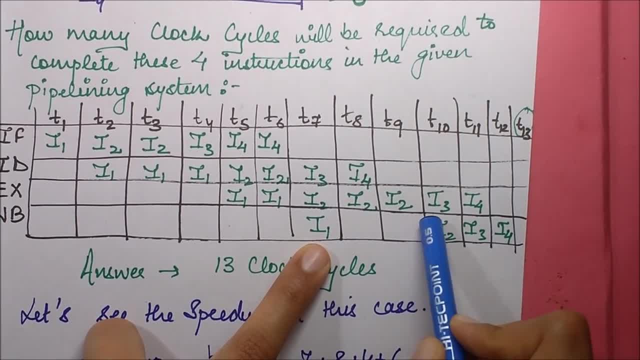 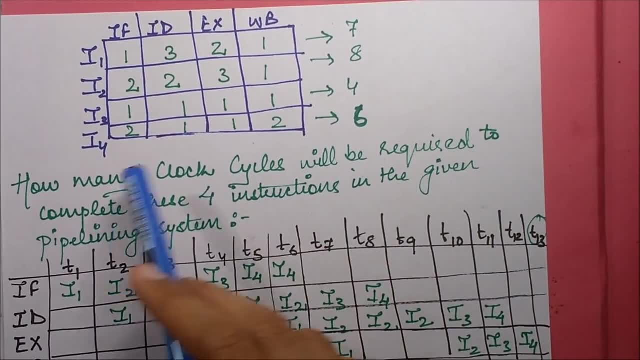 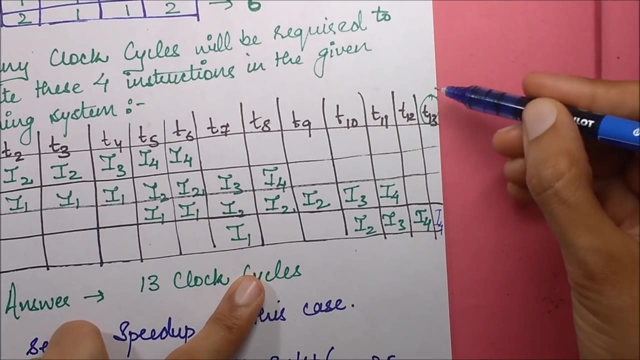 come here now. i2 cannot come here because i2's execution has completed over here. so i2 will be coming over here, then i3 and then i4. now i4 takes how much for? uh? two clock cycles for completion. so i4 has been written twice over here now so you can see the entire thing has completed after 13. 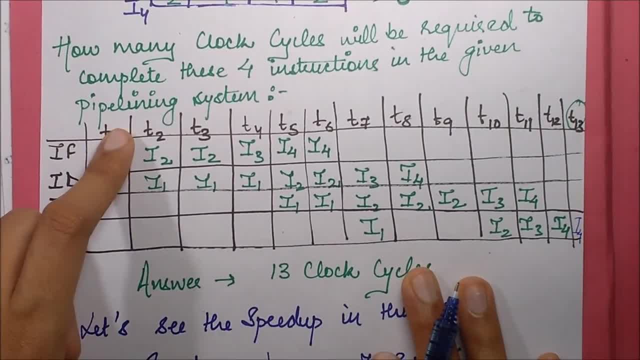 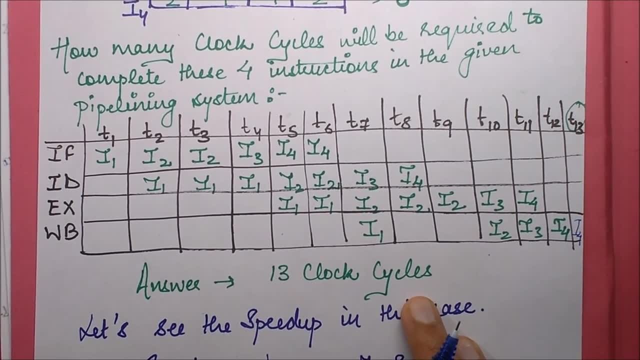 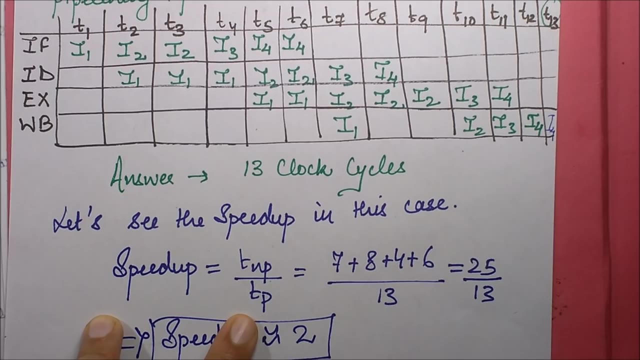 clock cycles. so the total time taken for the execution of this entire group of tasks is 13 clock cycles. right, so now we just finally compute the speedup, although it was not not asked in the question, but just for our understanding, we compute the speedup. what is the speedup? now? speedup will be what TNP? TNP is what total time taken in. 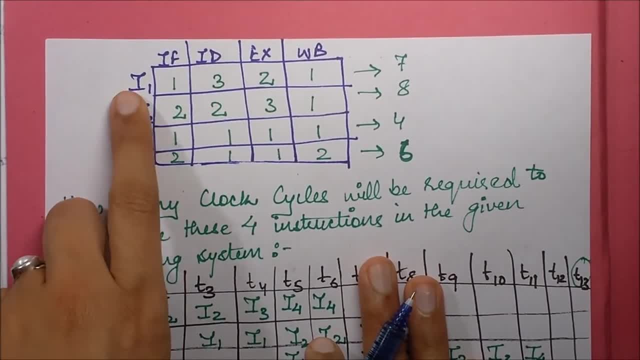 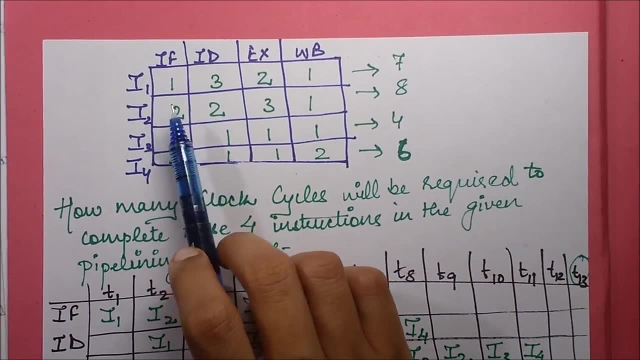 a non pipeline system. if this was a non pipeline system I would say: I 1 takes how much clock cycles? it would take 3 plus 2 plus 1 plus 1, which is 7. so we sum up the times of all the stages of this instruction. similarly for I 2.